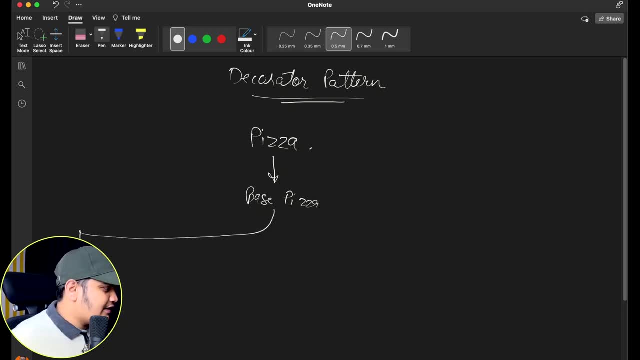 of pizza. So let's take the simple example. This is the same example that you will see everywhere when we are Y hadn't seen anything like that. So you are going to have the vegetable pizza, So you need the vegetable pizza. right, You can have a vegetable pizza. Add some extra cheese. You need군 brought. 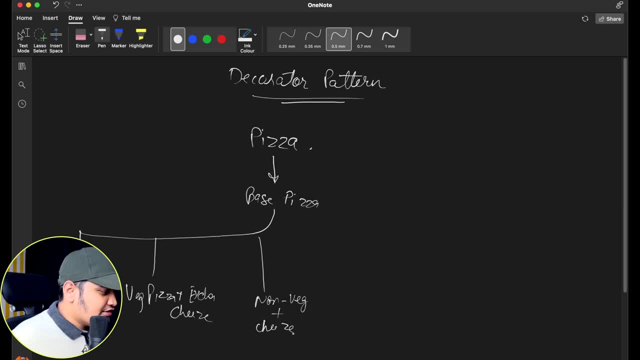 in the book ofippichgio. You can have nonveg pizza, Add cheese. Next, we need more caolpino. You need the vegetable pizza. Add some extra mushrooms and add extra cheese, Then add extra tomatoes. You can have a number of different toppings available and based on all these different toppings, you can 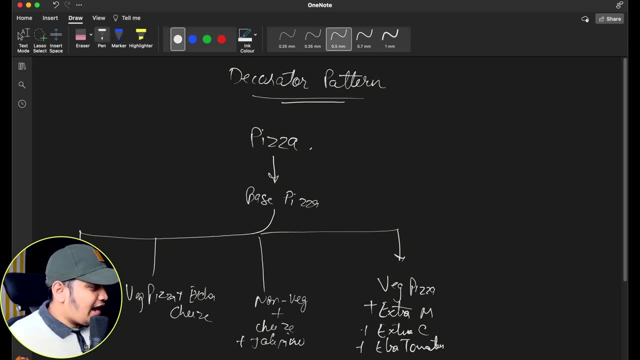 create the different pizza. but you can see that for this, I am creating a lot of different classes here, right, that is not ideal. when we are working with the application, when you are working with the object oriented programming, it is not feasible to have a lot of different. 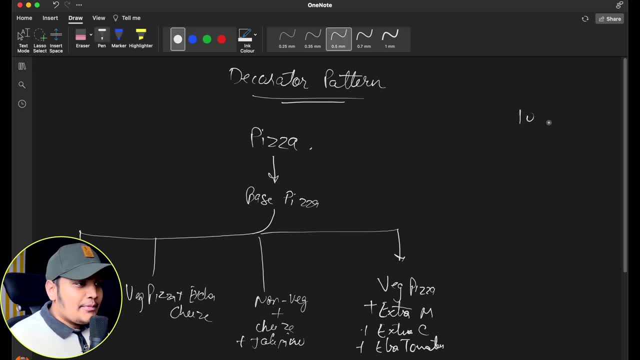 classes for the same reason. right, you can see, if you have 10 different toppings available, right then, how many classes that we will create. there is a lot of permutations and combinations available, so it is not feasible, so we need to come up with an approach that we can use. 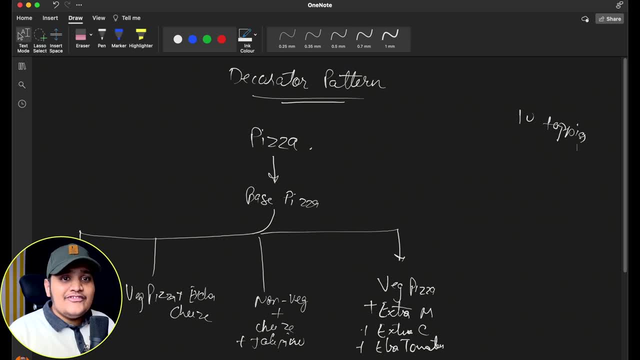 all those different behaviors, all these different classes, and we can create a different behavior. we can add the different behavior on top of the existing class itself. So if I have the pizza and if I add extra cheese, that itself will return me the pizza. that itself is a pizza, but with extra behavior on top of that. if I add extra tomatoes and 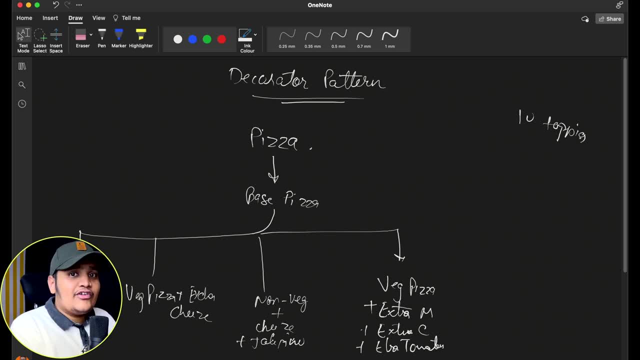 itself It's a pizza, but with another behavior. If I add another extra cheese, right, then it's again a different behavior, but but with the same class, the same pizza. So you can see that it is just changing the behavior, but the base class is the same. 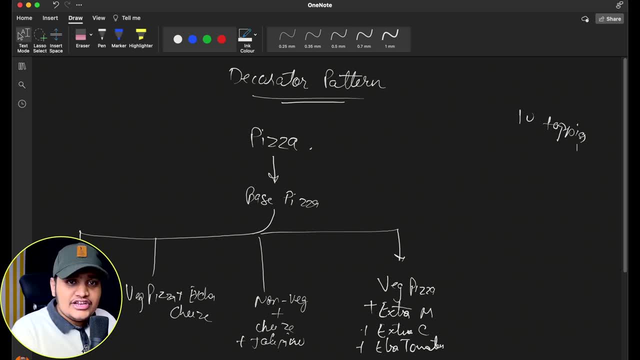 So how we can achieve this? like we can convert or we can change the behaviors, but the base is always the same. It will return the same thing. Okay, So for that we can use the decorator pattern. So decorator pattern will allow us to decorate any of the particular class. 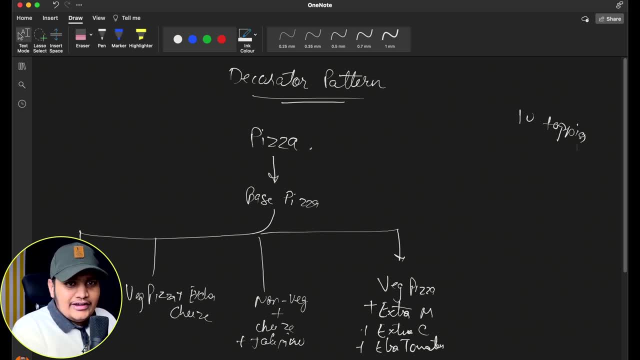 It's like adding the toppings on top of the pizza, right Like? you have the pizza, you will decorate it and you will add some toppings On top of that. you will decorate it and you will add some more toppings On top of that. you can again decorate it. That is, adding some more toppings. 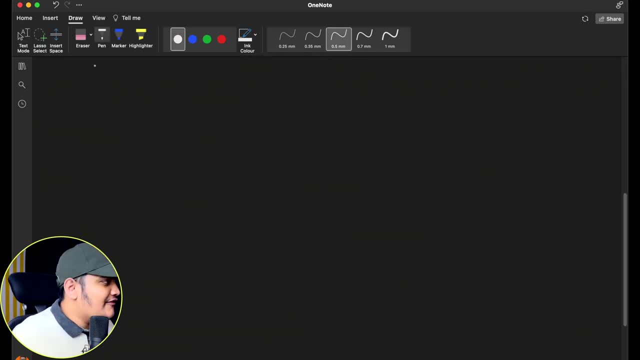 Okay, So let's understand how we can achieve this. So what we will have is we will have the pizza class available here, pizza interface: Okay, And this is going to be the interface. So anyone can implement this interface here. So it will have the method. 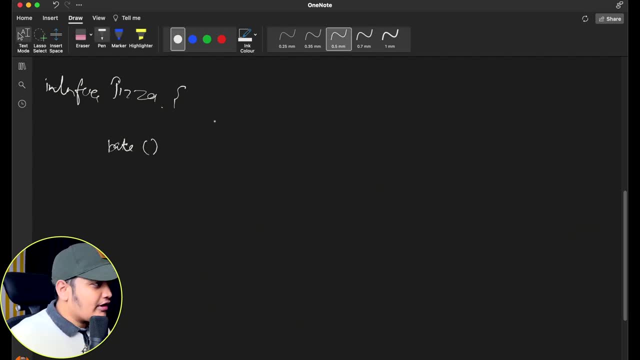 Suppose it has a bake method that we need to bake the pizza. Okay, So suppose there is a base pizza class available. This is a base pizza which will implement pizza here, And it will have the bake method implemented. Okay, This is the base class. now. 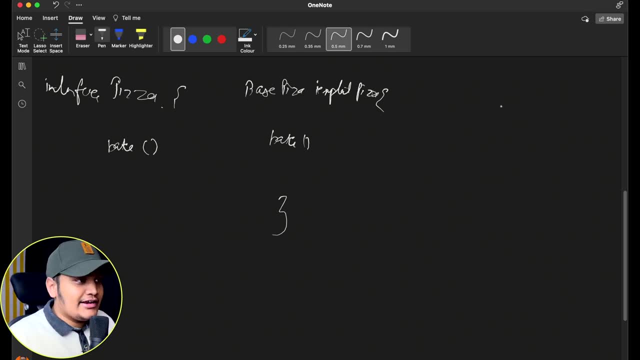 Now suppose I want to have the decorator. So what I will do? I will create a pizza decorator class. So I will create a pizza decorator class, pizza decorator which is going to implement pizza right, Because at the end it is a pizza, And what I will do is this: pizza decorator. 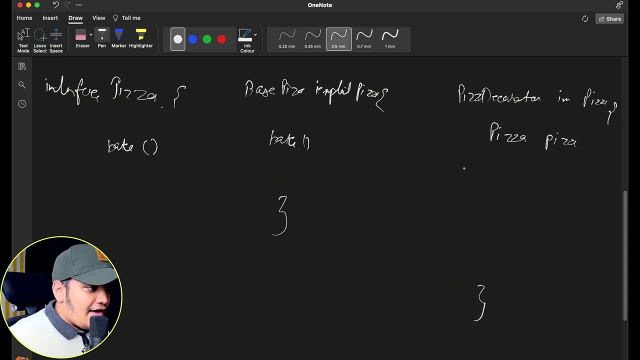 will have the instance of pizza class And we will have a constructor And within this constructor we will pass the interface. We will take the pizza interface. I just take a pizza interface. Huh, no pizza space Here. And whatever the PISA interface we pass, we will assign it over here. 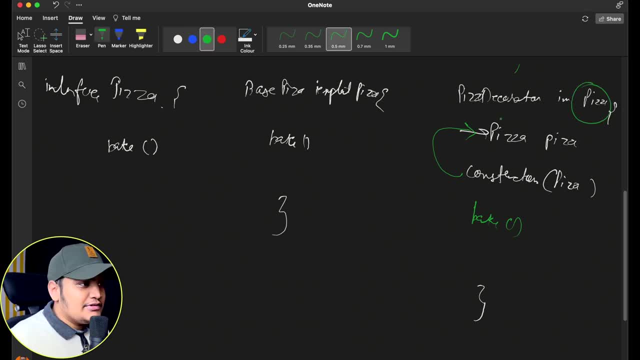 Okay, From the construct of tornar of $100 over here, And it will have the bake method also. right, Because we need to implement the big metric which is coming from the PISA interface. Okay, now this PISA decorator can be extended. 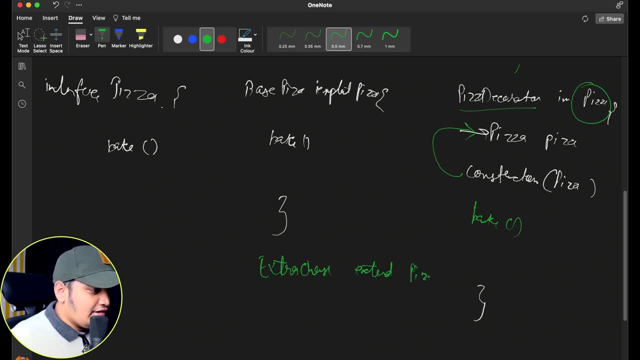 It can be subclassed by multiple. So suppose if we have extra cheese, right, So extra cheese, Okay, also will have the object of a pizza and it will add the pizza over here using the constructor and within the bake method it will add pizza. whatever the super class will have plus extra. 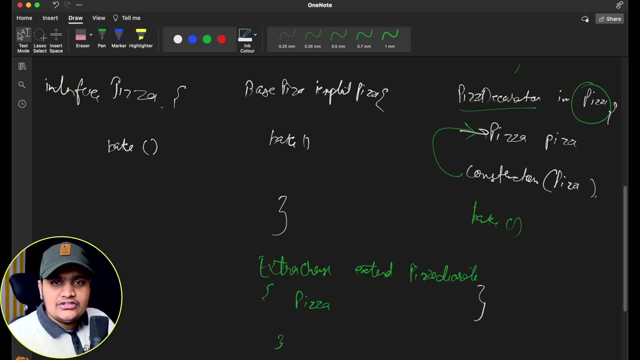 cheese. similarly, if we have extra mushroom, then this is also. that is also going to extend the pizza decorator and it is going to add extra mushroom in the bake method. so you can see that all this decorator are nothing but a same returning pizza, but adding some of 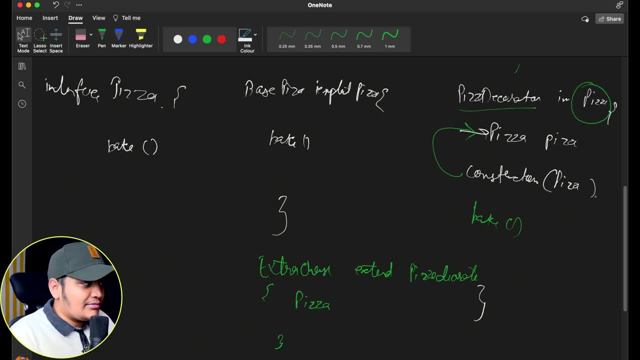 the extra behaviors to the bake method which we have extended from the pizza itself. okay, so you can see that everything is similar. everything is returning the same thing here. so this way we can have the decorator implemented. it's just the same thing, like it is going to add, then return the same class available, but with a different behavior. so let's understand. 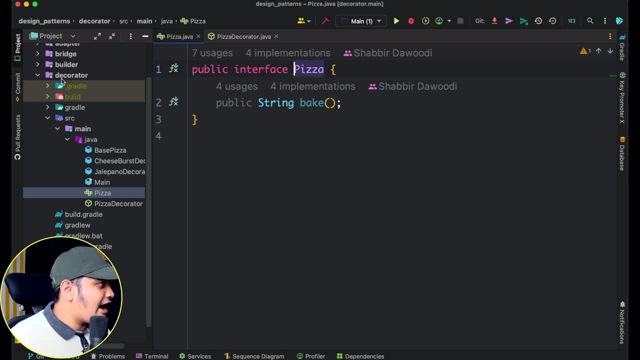 more with the code. so if you go here, so here you can see that i have the decorator project available and within this decorator, you can see i have one interface that is a pizza. okay, and this pizza interface, you can see it has one method, that is the bake method. okay now. 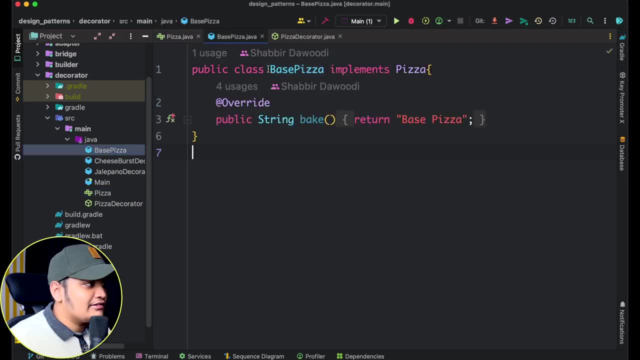 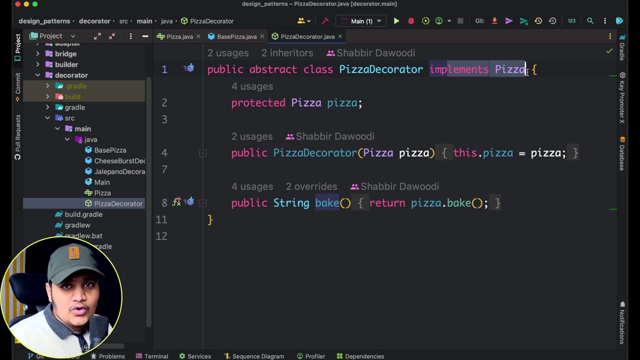 this pizza, you can see that it has been implemented by base pizza. okay, and we have implemented this bake method, which is returning the base pizza, simple thing. now you can see, i have created a pizza decorator class. this is an abstract class which is implementing pizza. okay, now you can see, i have the instance of 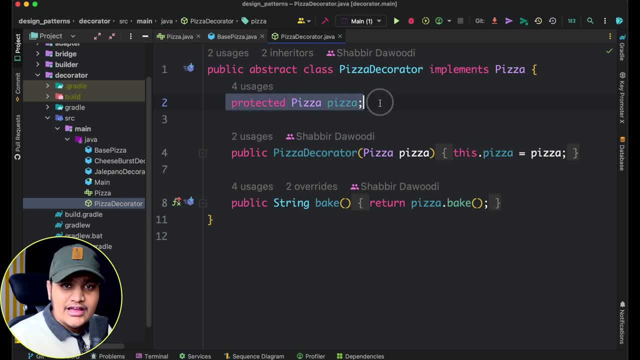 a pizza interface here. okay, so you can see i have the pizza interface and, using the constructor, i am assigning the object reference here. so whenever, whatever the pizza i am passed by passing here from this constructor method, i have that object and as we have implemented pizza, i have to override the bake method and you can see that within the bake method i. 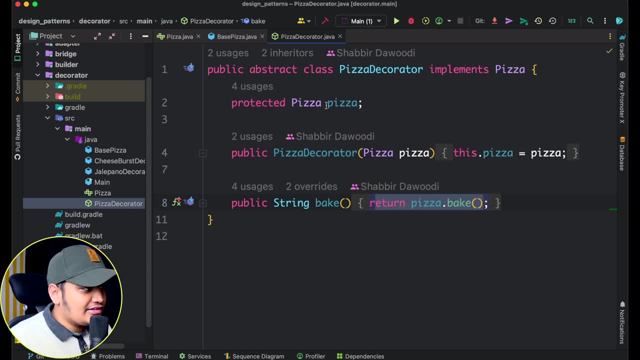 am just returning the pizza dot bake. so whatever this method, whatever this object is, that's bake method i am returning now. this class is going to be implemented by the different decorators we have. so you can see we have the jalapeno decorator. okay, this jalapeno. 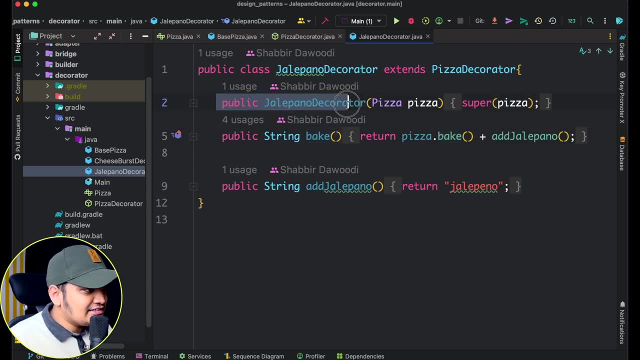 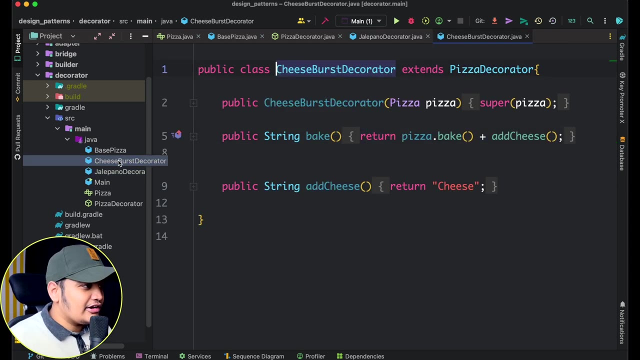 decorator, you can see that it is extending pizza decorator. it has the constructor which is taking the pizza object, as we seen in the pizza decorator and within this bake method, you can see that it is returning the pizza plus add jalapeno right. similarly, if you go to the cheese bus decorator, it is 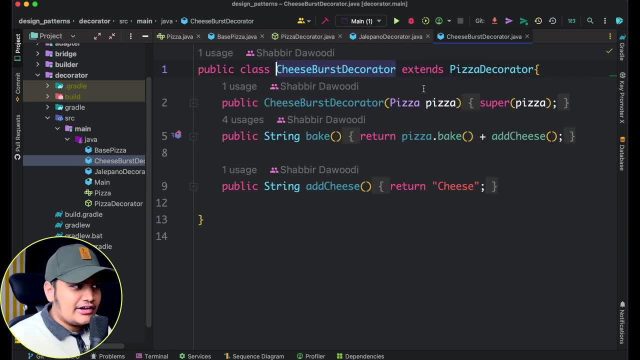 cheese bus decorator, right, and which is extending the pizza decorator. it has the constructor and in the bake method you can see it is returning pizza dot bake plus add cheese, this add cheese method. okay, so you can see that we have the n number of decorators available and at the 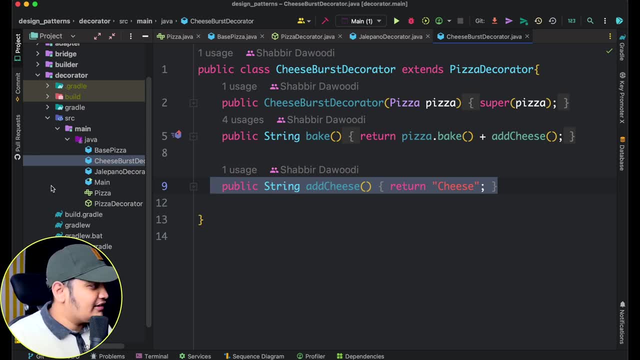 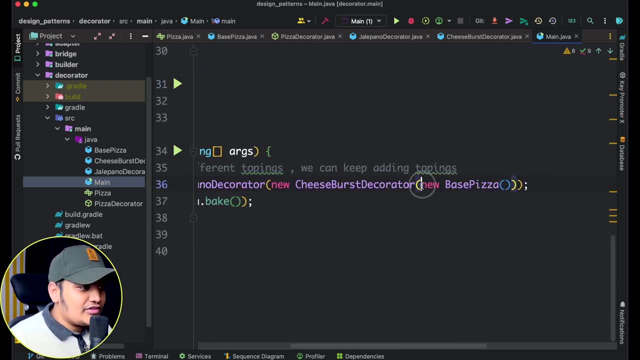 end, it will return the same thing. okay, so now how we can call this? so for calling, if you go to the main class here so you can see that i want pizza, i want pizza from what? i want pizza from base- okay, main base. now that main base, i can decorate it. okay, i want to add the cheese burst: okay, pizza. so this: 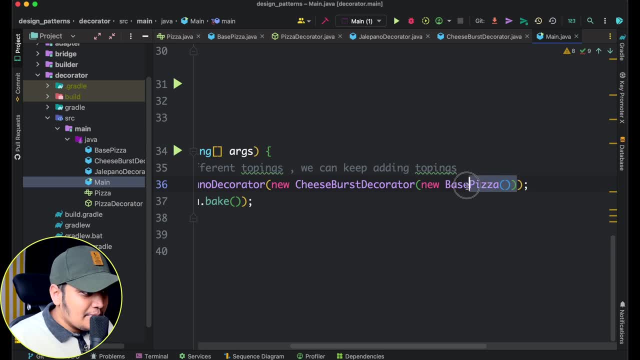 you can see that this base pizza is decorated by the cheese burst decorator. you can see that this is the decorator on top of the base pizza. okay, now, on top of that cheese burst decorator, you can see that this is decorated by the jalapeno as well. so that entire thing is now. 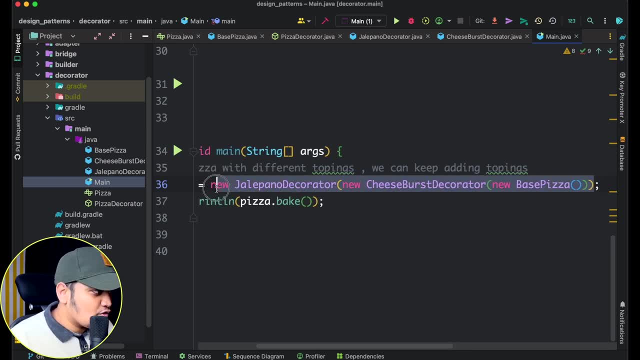 again, you can see is decorated by the jalapeno decorator. okay, so you can see that on top of that, again, it is a jalapeno decorator, but at the end, jalapeno decorator is implementing the pizza interface, so at the end this is going to return pizza itself. okay, so if i 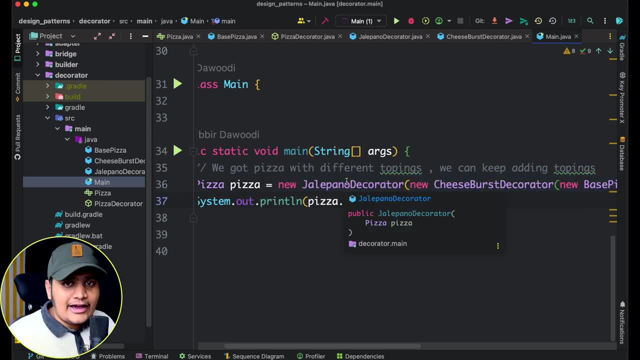 want to again decorate with something else, i can again, on top of that, decorate that particular class. so you can see that this is going to return pizza plus, this is also going to return the pizza plus this is also going to return the pizza itself. okay, so everything is going to return pizza, so we have the pizza object and we can bake. 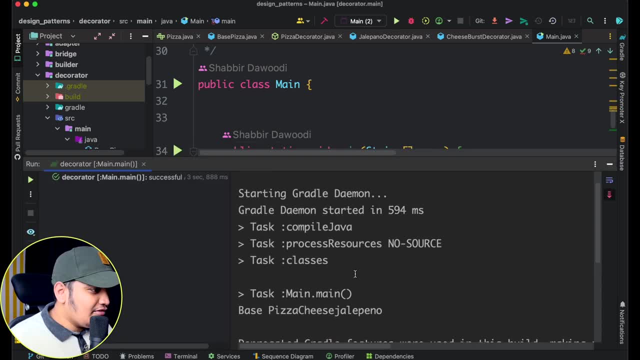 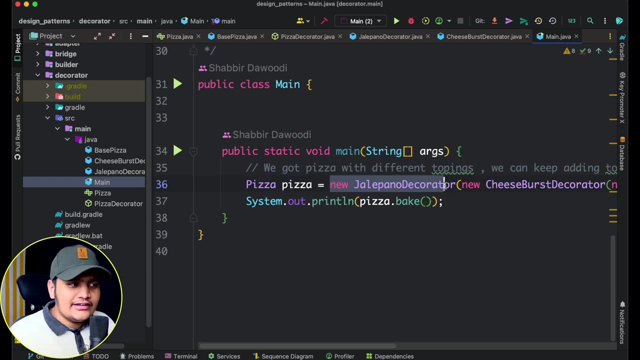 the pizza object. so if i run this, so you can see that i am getting the base pizza cheese and jalapeno. so this way you can see that we can add the different decorators based on the different classes that we have. okay, so we can create n number of decorators and you can see it's. 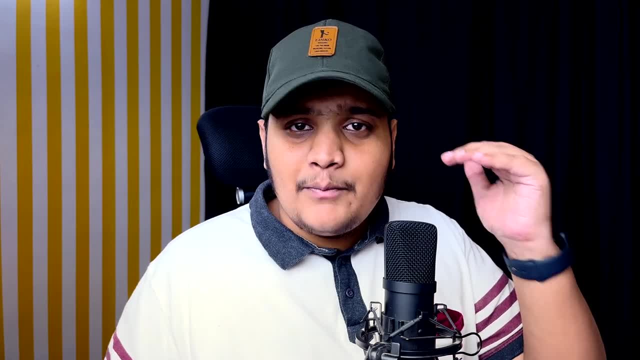 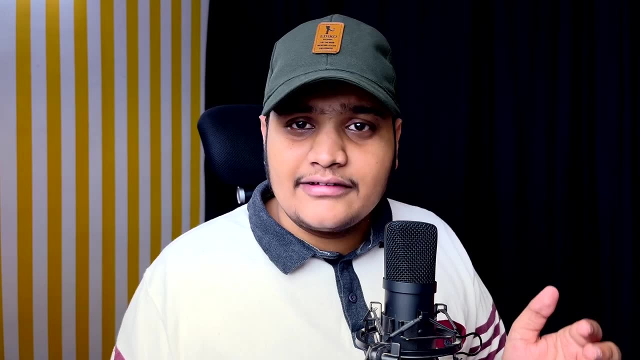 really easy to implement. what you have to do is you can have the base class ready and you have the different decorator which is implementing that base interface and it has the object of the same thing and you can always have those methods and written the same thing and within the 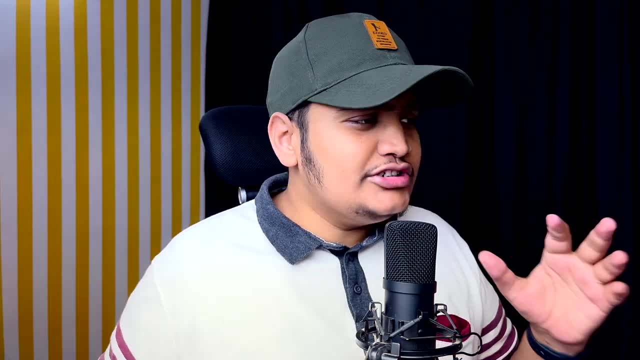 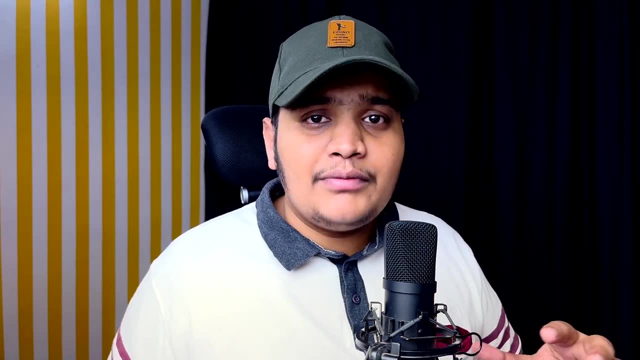 constructor, you have to take the same base class object. So this is also really simple structural design pattern to implement and if you are asking the interview, you can go ahead with the simple example. if not the same example, you can always prepare your particular example before interview and that you can explain in your interview. 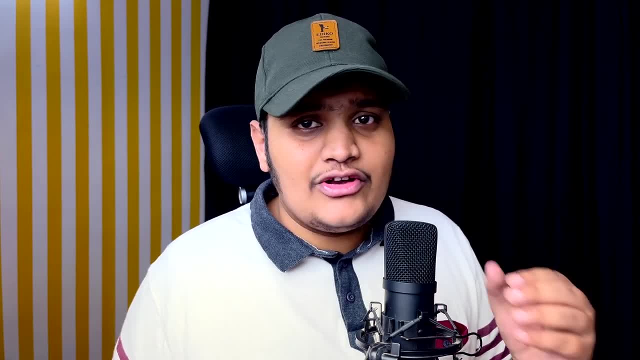 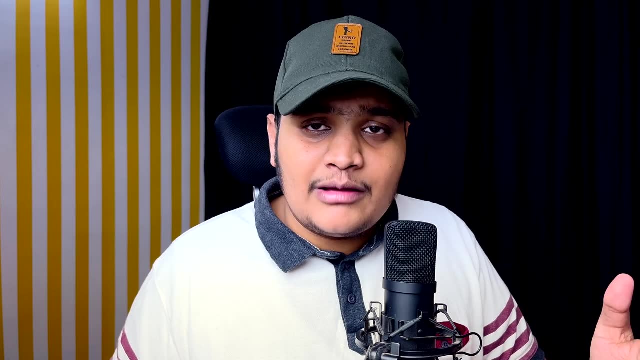 process. Okay, make sure that you have a couple of different examples ready when you're going for the interview. if you are explaining any design pattern with one of the example, if interviewer may ask like give me some other example or real-world example, you can go ahead. 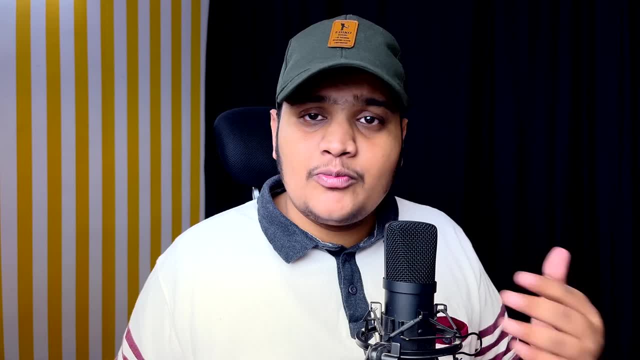 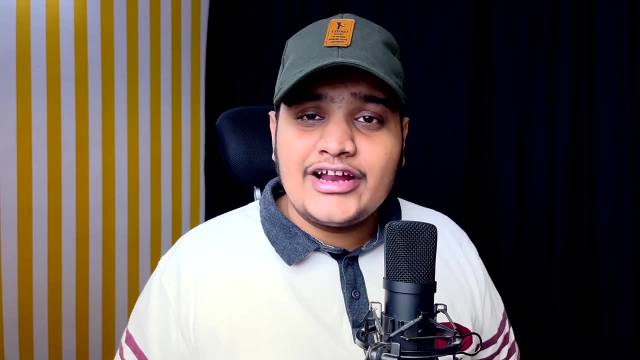 with that approach as well, if you have prepared for it. Okay, so make sure that you prepare different examples for a different design patterns. So that was all about the decorator design pattern from the structural design pattern type. if you have any doubts regarding any of the things that we have covered, then do.